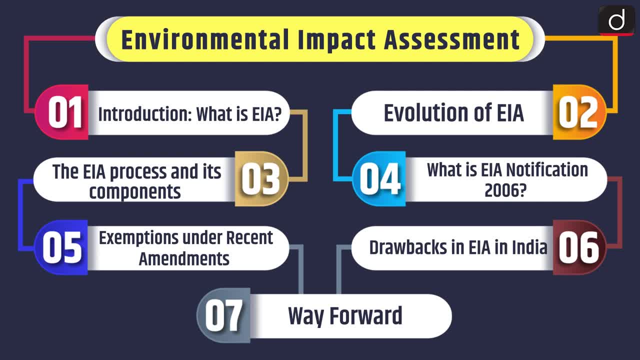 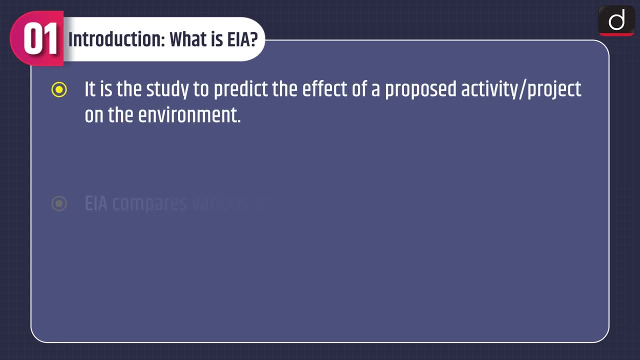 EIA, the EIA process and its components. what is EIA? notification 2006,, exemptions under recent amendments, drawbacks in EIA in India and way forward. First of all, let's discuss what is EIA. It is the study to predict the effect of a proposed activity or project on the environment. 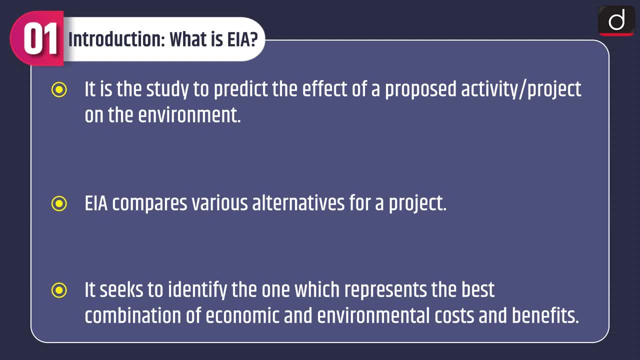 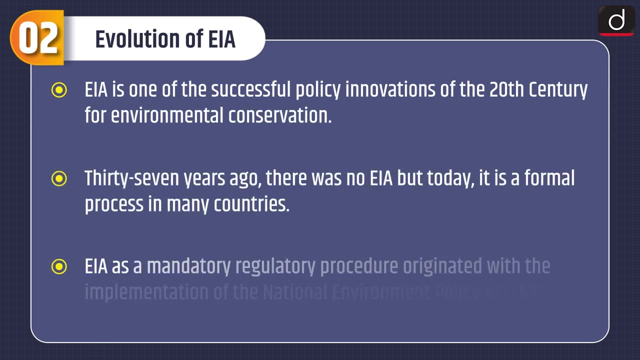 EIA compares various alternatives for a project. It seeks to identify the one which represents the best combination of economic and environmental costs and benefits. Now moving on to evolution of EIA. EIA is one of the successful policy innovations of the 20th. 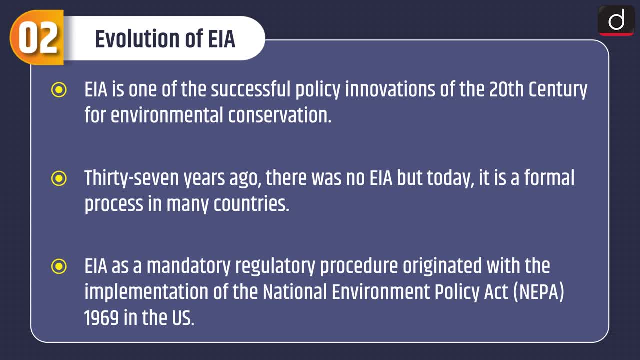 century for environmental conservation. 37 years ago there was no EIA, but today it is a formal process in many countries. EIA as a mandatory regulatory process originated with the implementation of the National Environment Policy Act, or NEPA, 1969 in the US. 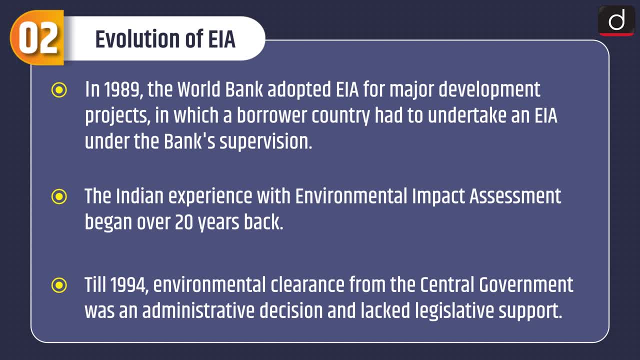 In 1989, the World Bank adopted EIA for major development projects in which a borrower country had to undertake an EIA under the bank's supervision. The Indian experience with environmental impact assessment began over 20 years back. In 1994, environmental clearance from the central government was an administrative decision and 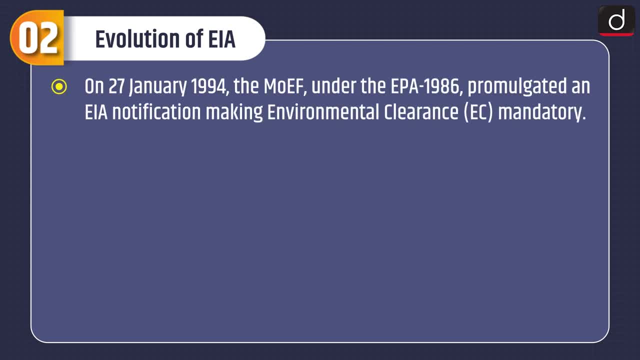 lacked legislative support. On 27 January 1994, the MOEF, under the EPA 1986, promulgated an EIA notification making environmental clearance. Certain activities permissible under the Coastal Regulation Zone Act 1991 on EIA were to be legalized under the National Environment Policy Act. EIA was the first government to be able to terminate EIA's direct activities that were unlawful to the public. It was the only one to have access to the EIA and NEPA license or EIA's EPA license. The first has to be expired before it isינ chak pompa in the next issue, and the second to have application. The last has to be expired before it is cancelled. The third has to be expired before it is cancelled. The third has to be expired before it is cancelled. The fourth has to be expired before it is cancelled. The second has to be expired before it is cancelled. 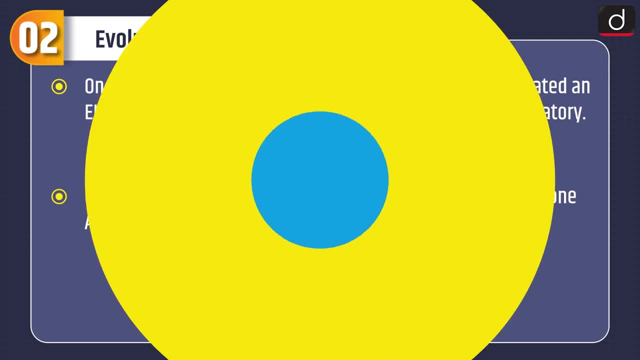 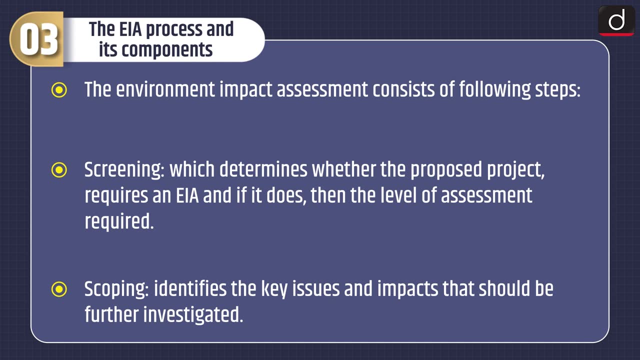 also requires similar clearance. Now let's discuss about the EIA process and its components. The environment impact assessment consists of following steps: Screening, which determines whether the proposed project requires an EIA and, if it does, then the level of assessment required. Scoping: identifies the key issues and impacts that should be further investigated. Baseline: 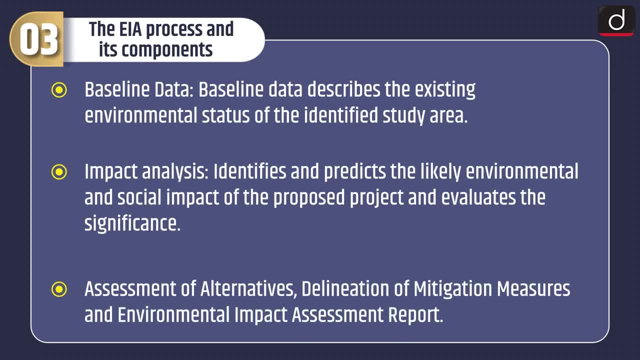 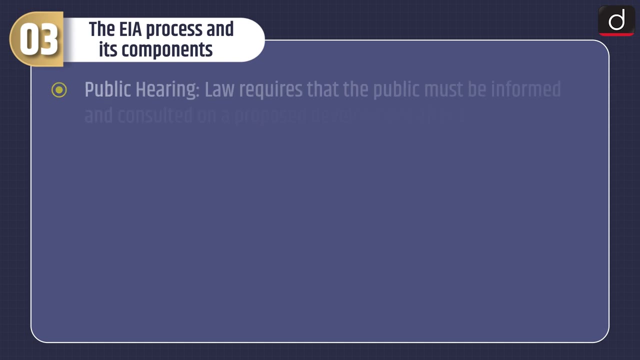 data describes the existing environmental status of the identified study area. Impact analysis identifies and predicts the likely environmental and social impact of the proposed project and evaluates the significance, Assessment of alternatives, delineation of mitigation measures and environmental impact assessment report. Public hearing Law requires that the public 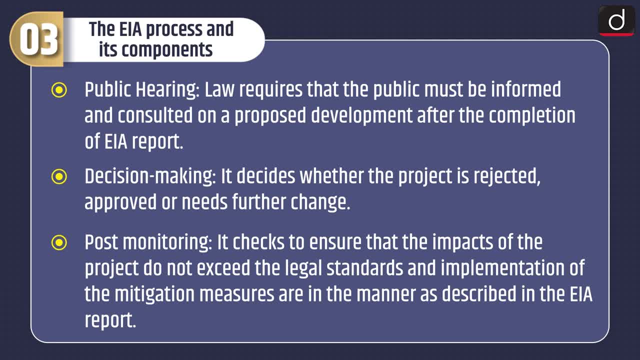 must be informed and consulted On a proposed development after the completion of EIA report. Decision making: It decides whether the project is rejected, approved or needs further change. Post monitoring: It checks to ensure that the impacts of the project do not exceed the legal standards and implementation of the mitigation. 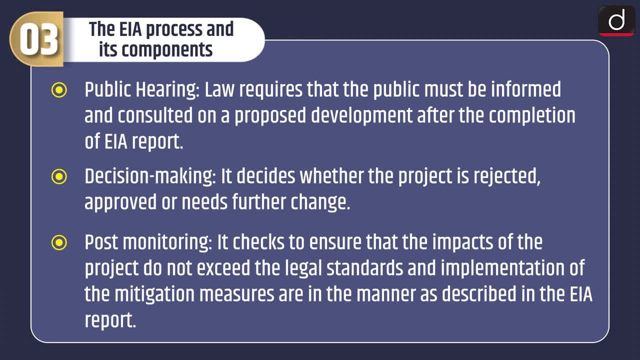 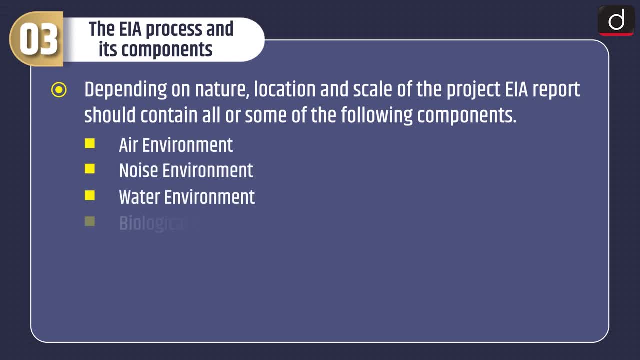 measures are in the manner as described in the EIA report, Depending on nature, location and the project. EIA report should contain all or some of the following components: Air environment, noise environment, water environment, biological land, socio-economic and health environment. 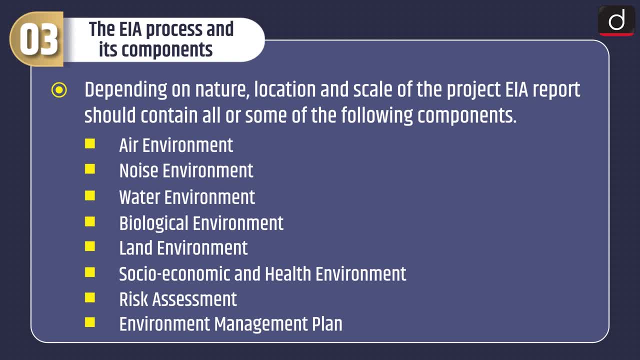 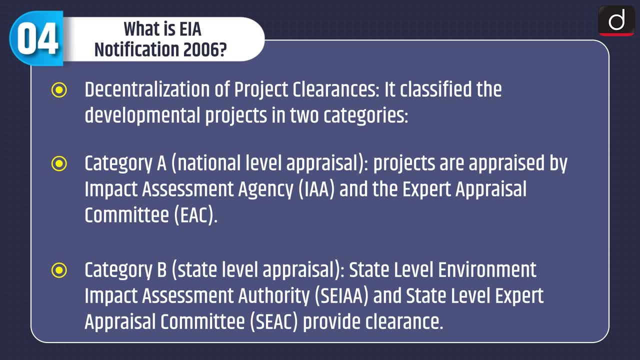 risk assessment and environment management plan. Now let's understand what is EIA notification 2006.. Decentralization of project clearances. It classified the developmental project. There are two categories. Category A: national level appraisal Projects are appraised by impact. 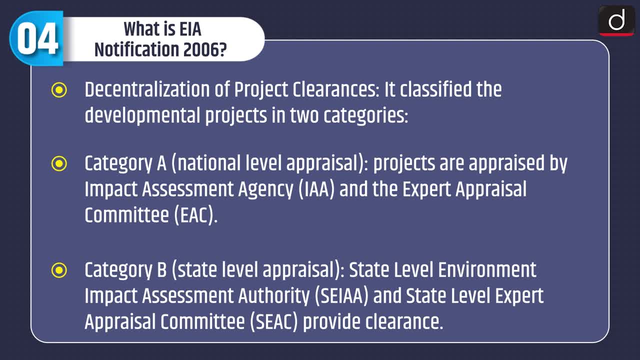 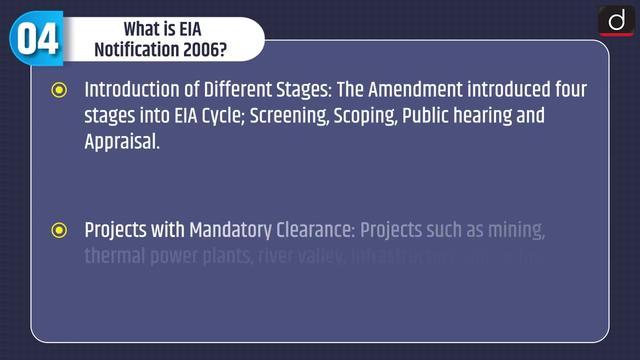 assessment agency, or IAA, and the expert appraisal committee that is EAC, And category B, that is state level appraisal. State level environment impact assessment authority, or SEIAA, and state level expert appraisal committee, or SEAC, provide clearance. In addition of different stages, the amendment introduced four stages into the EIA cycle. 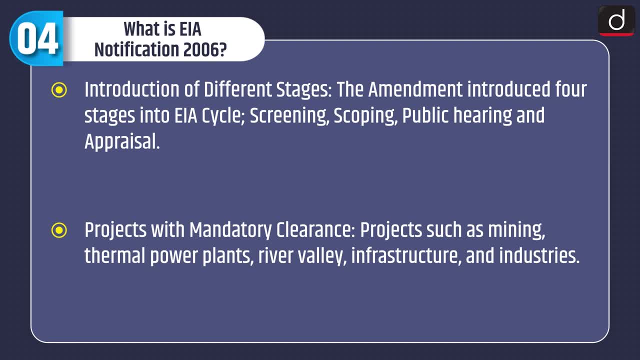 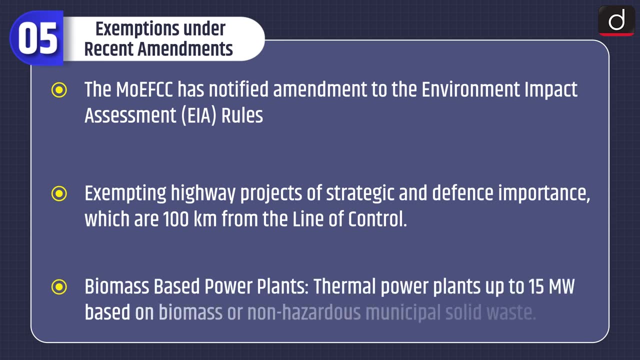 Screening, scoping, public hearing and appraisal, And projects with mandatory clearance, Projects such as mining, thermal power plants, river valley infrastructure and industries. Now moving on to exemptions under recent amendments: The MOEFCC has notified amendment to the environment impact assessment rules. 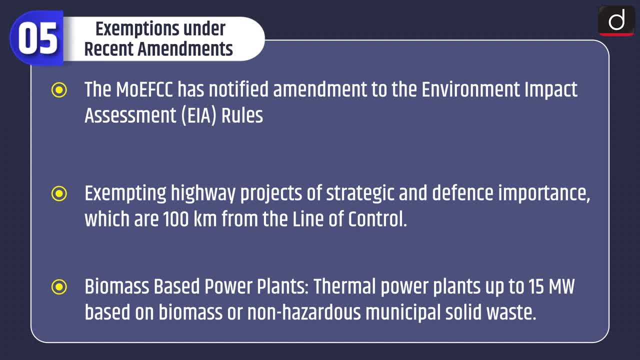 Now moving on to exemptions under recent amendments. The MOEFCC has notified amendment to the environment impact assessment rules Notifies both urban development and industrial level response Exempting highway projects of strategic and defense importance which are 100 kilometer from the line of control. biomass-based. 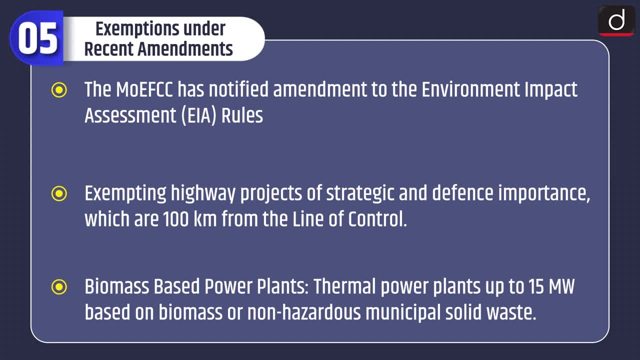 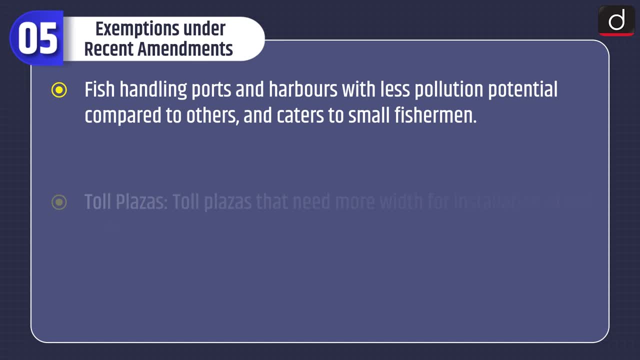 power plants, thermal power plants up to 15 Megawatt Based on biomass, or non-hazardous municipal solid waste Fish handling. ports and harbors with less pollution potential compared to others and caters to small fisherman Toll plazas that need more width for installation of toll collection booths. 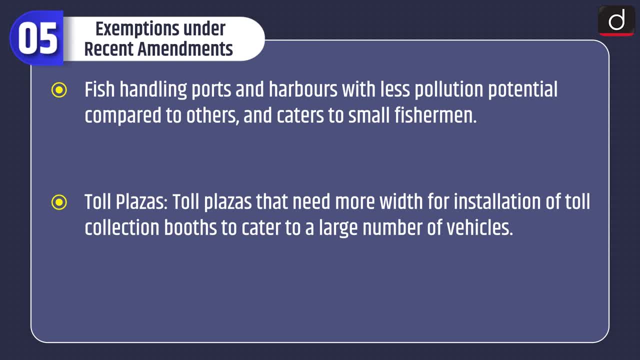 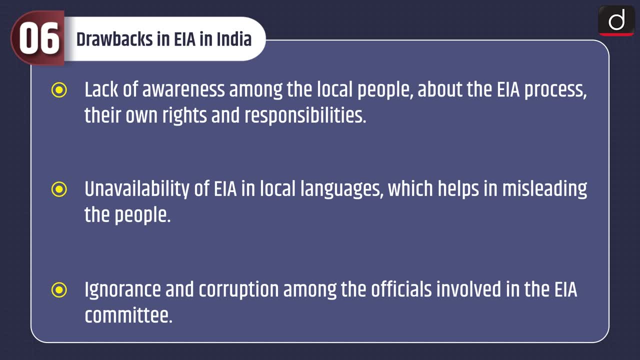 booths to cater to a large number of vehicles. Now let's discuss about the drawbacks in EIA in India: Lack of awareness among the local people about the EIA process, their own rights and responsibilities. Unavailability of EIA in local languages, which helps in misleading the people. 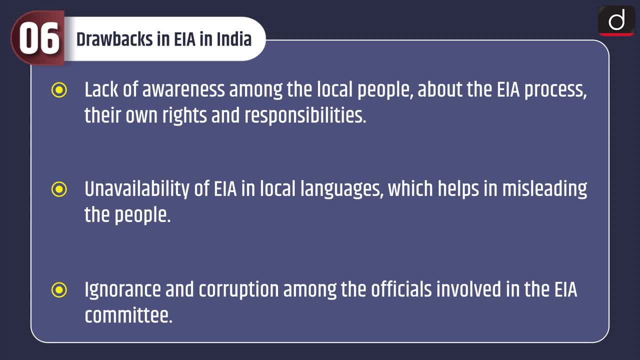 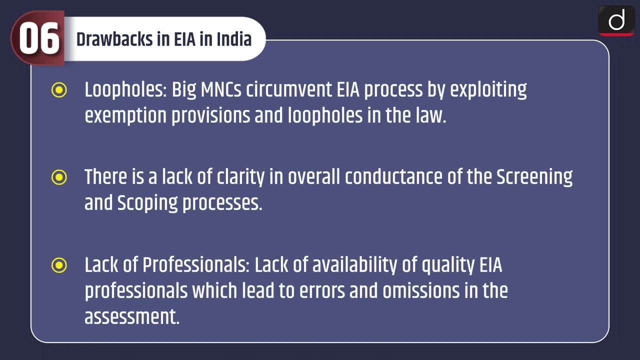 Ignorance and corruption among the officials involved in the EIA committee. Loopholes: Big MNCs circumvent EIA process by exploiting exemption provisions and loopholes in the law. There is a lack of clarity in overall conductance of the screening and scoping processes. 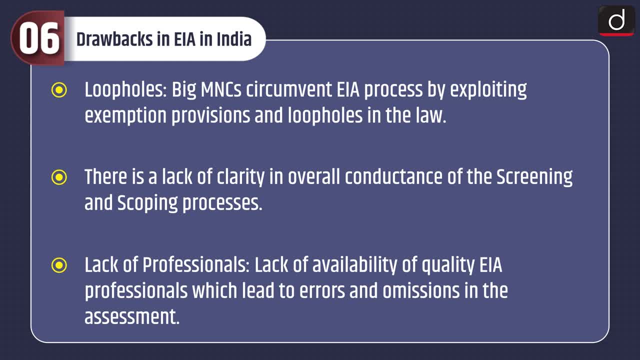 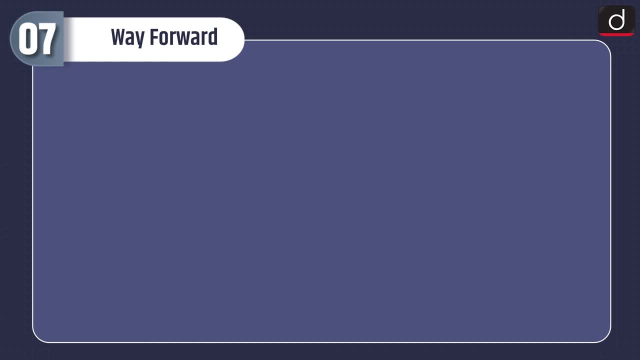 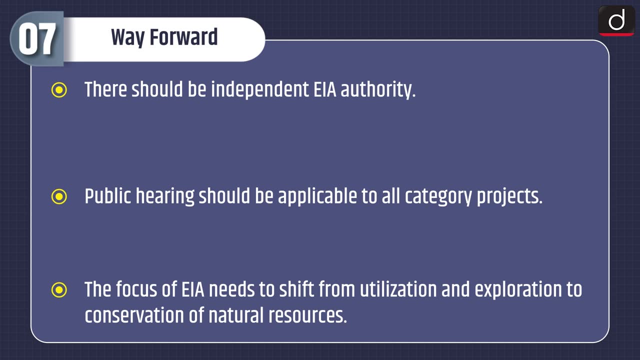 Lack of professionals, Lack of availability of quality EIA professionals, which lead to errors and omissions in the assessment. Now, lastly, let's discuss about the way forward. There should be independent EIA authority. Public hearing should be applicable to all category projects. The focus of EIA needs to shift from 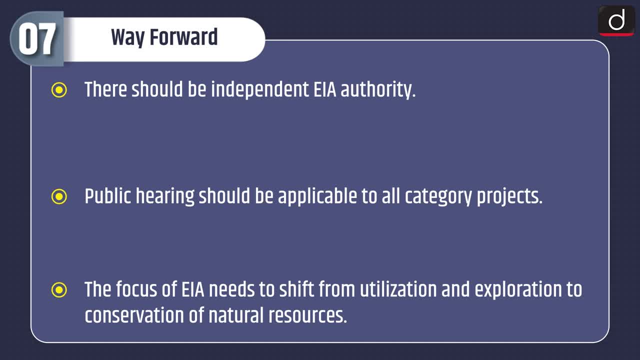 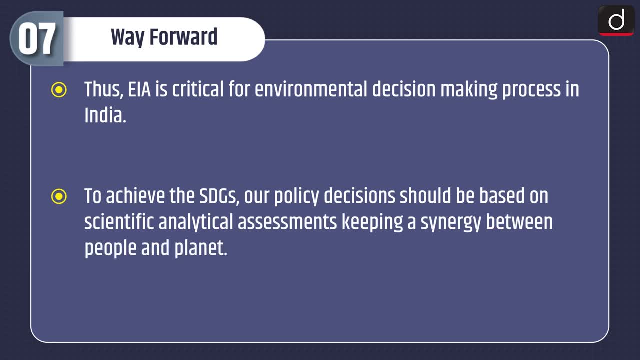 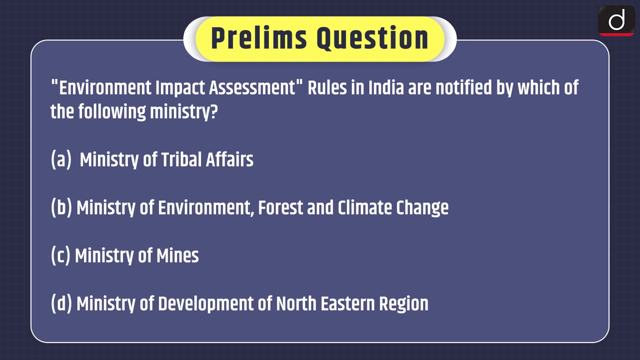 utilization and exploration to conservation of natural resources. Thus, EIA is critical for environmental decision-making process in India. To achieve the SDGs, our policy decisions should be based on scientific analytical assessment, Keeping a synergy between people and the planet. Now it's time for the practice questions. First of all, note down the prelims question: Environment.